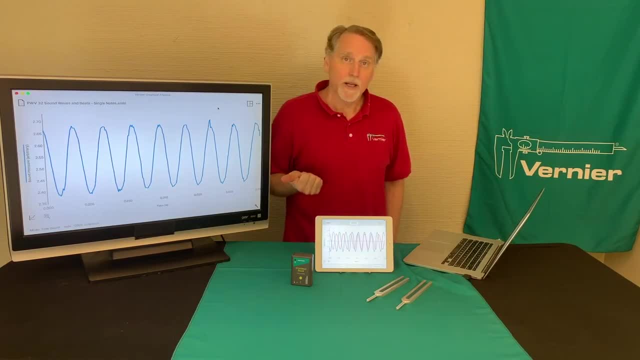 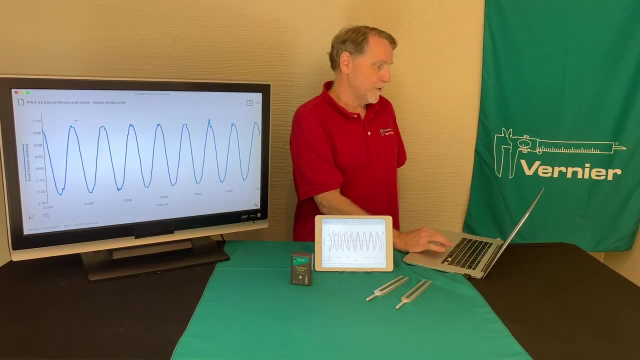 So there's some things you need to know. You need to know how to be able to get the time from it. You need to know how to be able to do some curve fitting So in order to get the frequency, the way you do, that is determine the period, and the period is the time it takes for, say, one wave to pass. 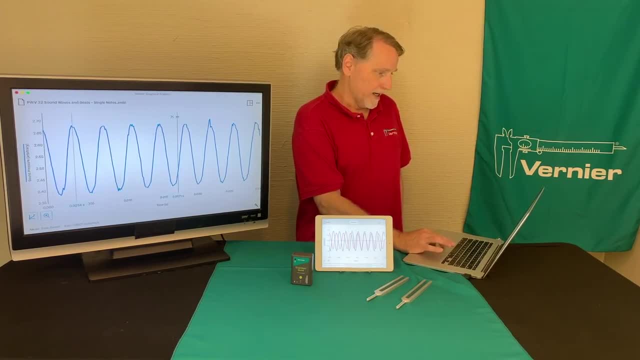 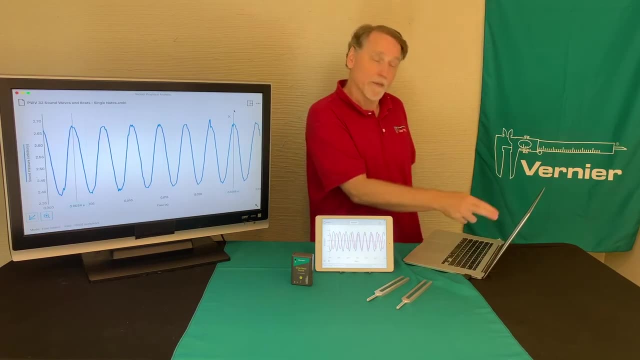 And a good way to do that is to actually highlight a number of peaks- I think that's six peaks- And from this I can get the actual time it takes to go for all six peaks. Then I can determine the time for one peak by dividing by the number of peaks there. 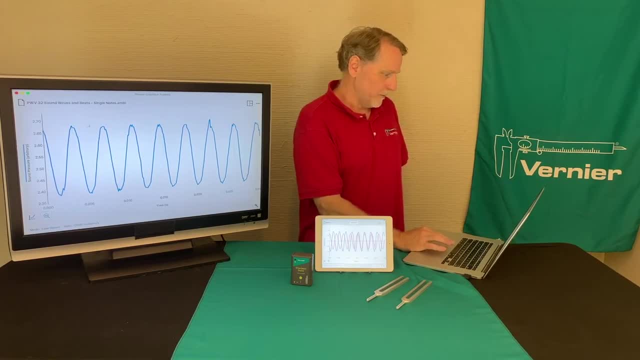 So you need to be able to do that one. The other thing you have to be able to do here is do a curve fit, And so I'll go down here, and the experiment asks you to do a sine fit, So I'll do that, and it gives you these values here. 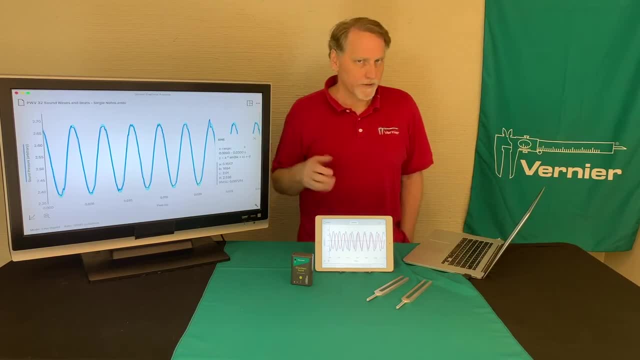 And so in the lab it refers to these Things like amplitude and frequency and how you work all that out there. So this is the first part of the lab. The second part of the lab is a different file And it is actually the one where the two sounds are recorded simultaneously. 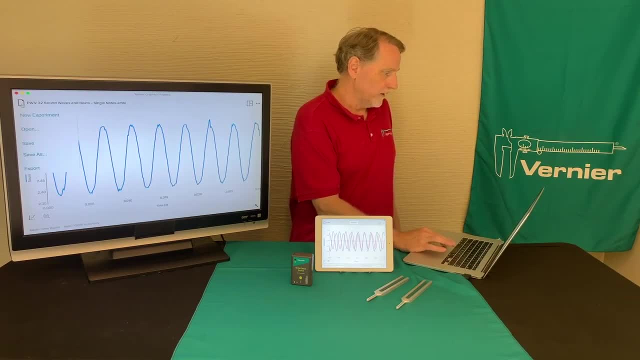 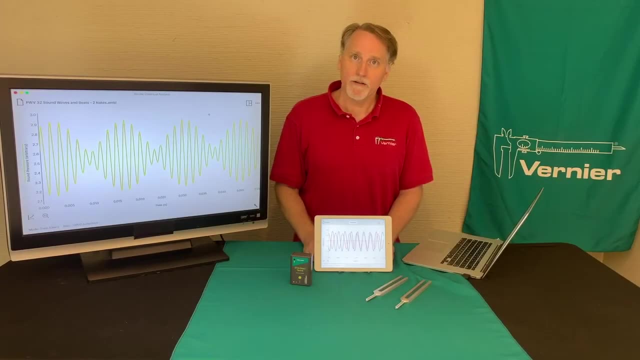 So I will do this. Let me open that file. So I'll open the file. I won't save that one. So I've opened the second file for the experiment, And this file is the one where the two tones were measured simultaneously. 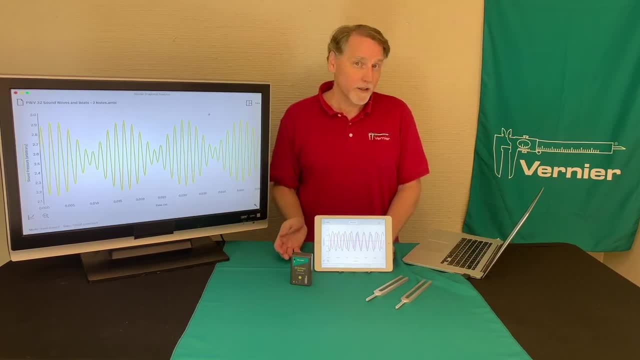 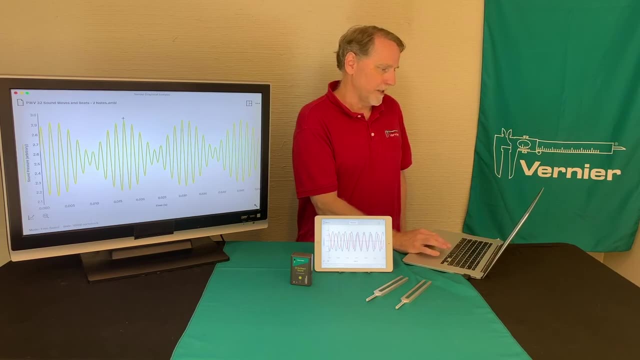 And that's why you get this pattern here. Like you did in the first part, you need to know how to be able to do the time, Because it asks you something about the beat frequency And the beat frequency is going to be like we did there. 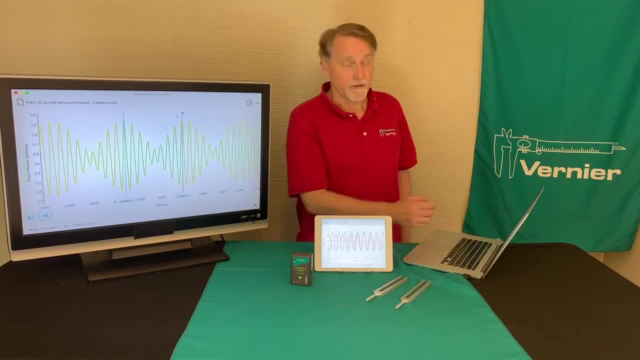 That would give you the period of the beat frequency And you take the reciprocal of that to actually get the frequency there. So that's similar to the first part there. So again, sound waves and beats. investigate sound using a microphone.